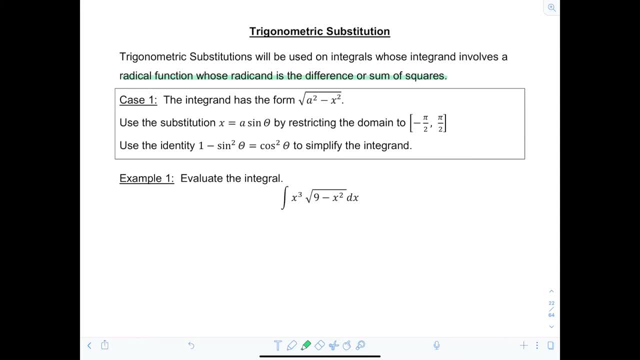 the primary function of them. So case one: if your integrand has the form rad, a squared minus x squared where a is a constant, then what you're going to do is use the substitution letting x equal a sine theta, and you need to restrict the domain to negative pi halves. 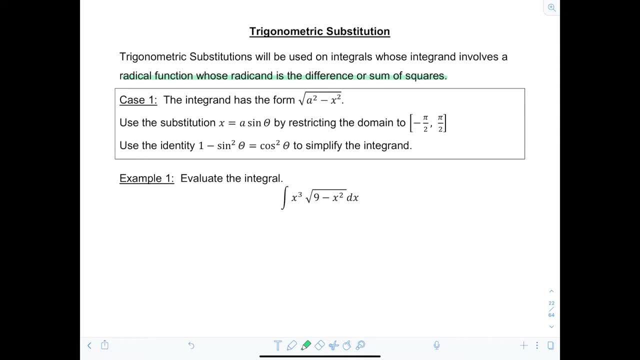 including that and pi halves. That way you're in quadrants one and four, restricting the domain on theta, and then you're going to use the identity one minus sine squared theta equals cosine squared theta to simplify the integrand. Okay, this will make a lot more sense once you see an example, so let's just dive right in. 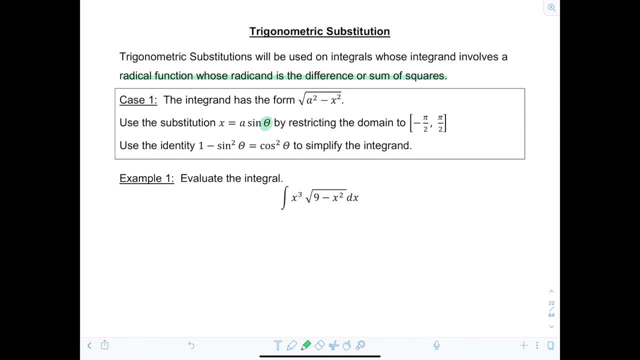 So we're going to evaluate the following integral. we've got integral of x cubed times radical nine minus x squared. Now you don't want to jump to trig substitution as your method of integration, right? When you first look at this thing you go: oh, could I use sub? 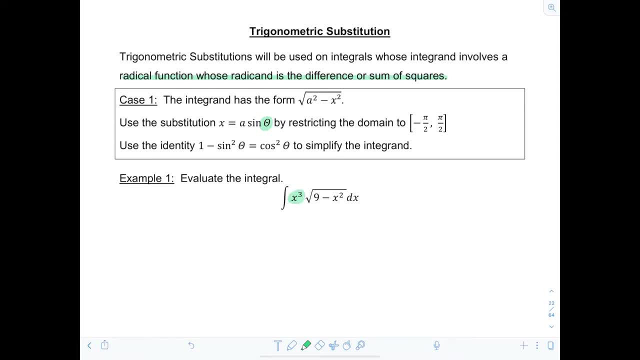 It's not looking like it because I've got an x cubed out here, not just an x. Maybe I could break it up, but that's looking a little messy. But notice here: this is a nice expression that we could use for a trig sub. So in this case a is equal to three, right, Since we have a squared. 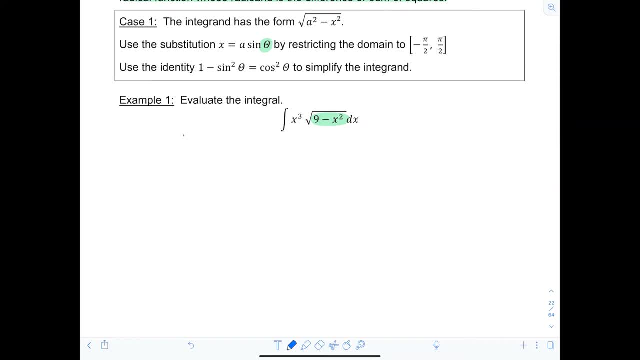 minus x squared. So what I'm going to do is let x equal three sine theta. all right, And now I have to change my whole integral so that it's in terms of theta. It's not like a u substitution, It's different. Then I'm going to find dx, So dx is going to equal three cosine theta, d theta. 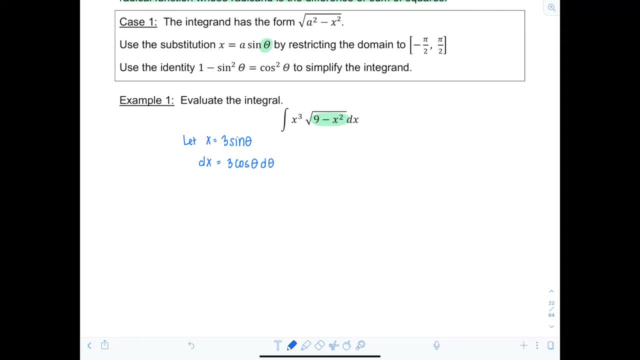 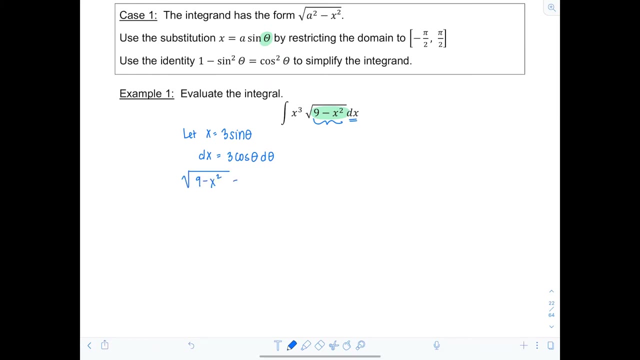 All right, So now I know what I'm going to replace dx with. Now let's figure out how the quantity underneath the radical is going to simplify, I have rad 9 minus x squared, and since I'm letting x equal 3 sine, 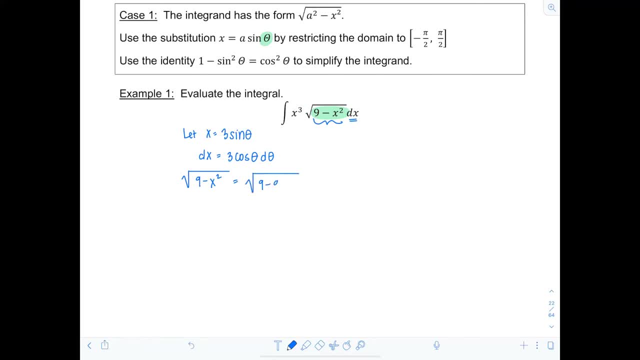 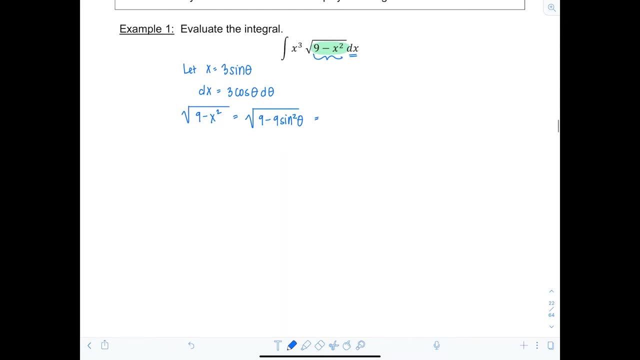 theta, that's going to be rad 9 minus 9 sine squared theta. All right, well, I can factor the 9 out from both of those quantities, so I'm going to have radical 9 times 1 minus sine squared theta. 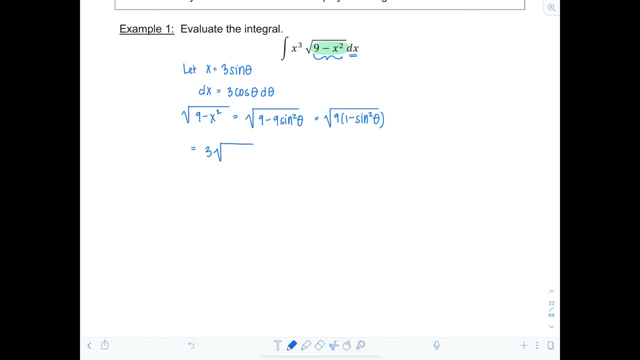 and this is going to give me 3 rad- cosine squared theta. And please be so, so careful when you have the square root of cosine squared theta, that's the absolute value of cosine theta. Do not forget those absolute value bars. Well, how do I know whether or not to use the radical? Well, I'm going. 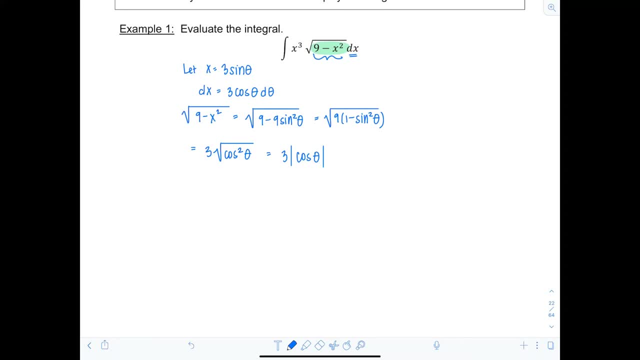 to use positive or negative cosine theta. Do I have to split this into two integrals? No, Remember, in this case, at the very beginning, we restricted theta between pi halves and negative pi halves, quadrants 1 and 4.. So in those quadrants cosine of theta is greater than or equal to 0,. 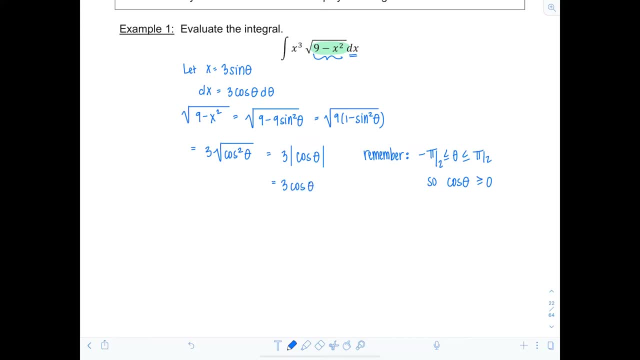 which means I know I'm just going to use positive 3 cosine theta, So that takes care of the quantity underneath the radical and the radical as well. right, We took the square root, So that's all taken care of there. dx, I have, that's right here. that's 3 cosine theta d. 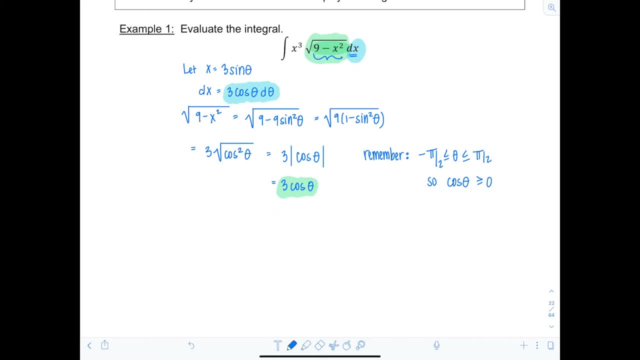 theta. Who's left? Yes, poor little x cubed. Okay, so x cubed is going to be 3 sine theta cubed, so that's going to be 27 sine cubed theta. So now it looks like everyone's accounted for. 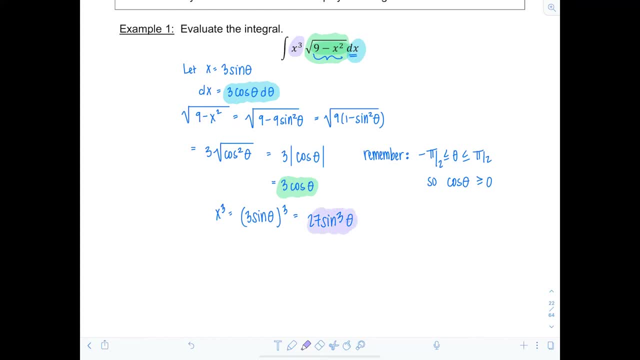 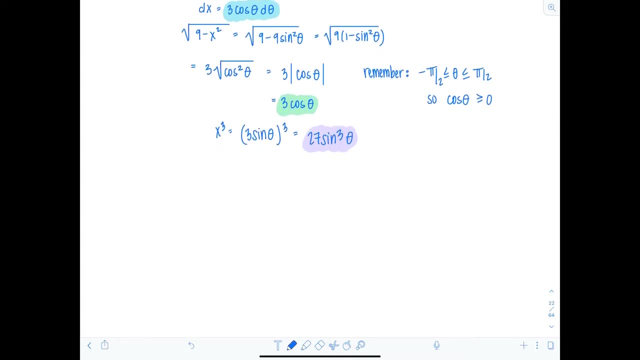 All right, x cubed is going to get replaced with 27 sine cubed theta. Okay, so here we go. Let's put it all together. I'm going to have integral 27 sine cubed theta times and the next piece is the rad 9 minus x squared. Well, that's replaced with 3 cosine theta. 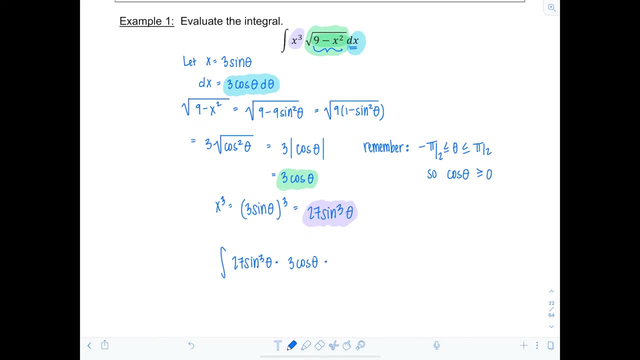 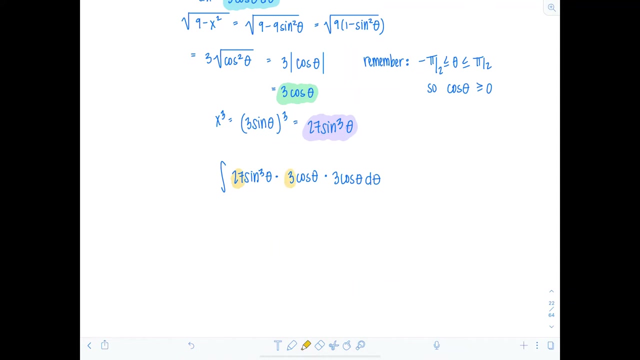 and then dx gets replaced with 3 cosine, theta, d theta, Fabulous, All right. as soon as I see an integral like this, I go: oh, we're taking all these constants outside, We don't need them harassing us, making a big mess. So 27 times 3. 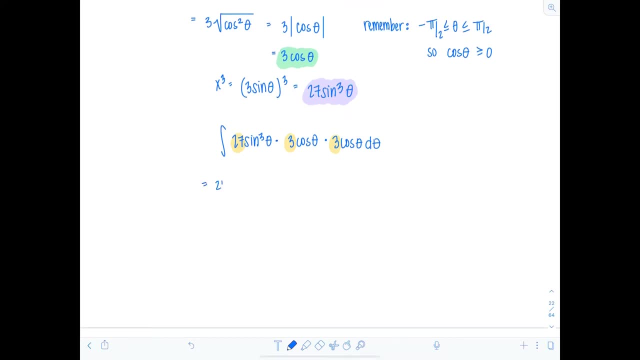 times 3, that's 27 times 9.. So we've got a 243 sitting out here, and then I have a sine cubed theta, cosine squared theta d theta. All right, now let's think back. Do we know how to integrate this expression? Why, yes, we do. We just did a whole lesson. 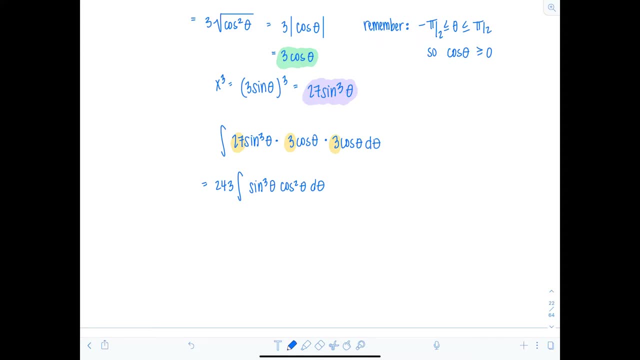 on trig integrals. Remember, when you have a product of powers, of sines and cosines, you factor out one of the factors on whichever trig function is raised to an odd power, right, You take the odd man out In this case, since sine is raised to the third power. I'm going to 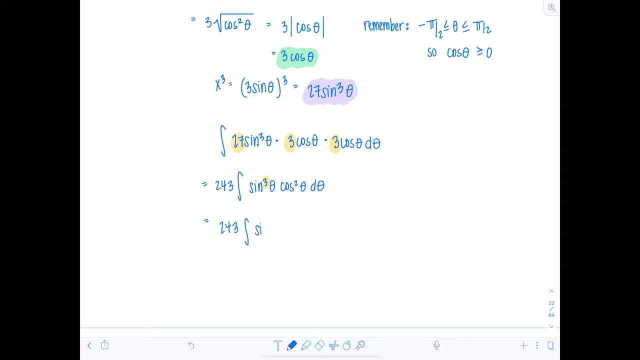 rewrite this as 243 integral sine squared theta Cosine squared theta times a sine theta d theta like that. All right, if you didn't watch that video yet, I'll link it up here. It's one of the very first cases we consider: Okay, why do we? 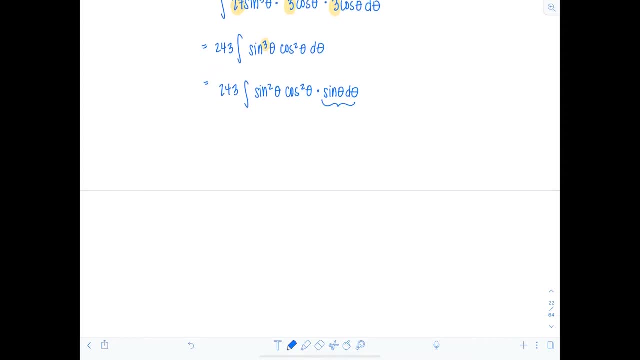 pluck off one of the factors of sine Because, remember, we want this sine theta d theta to get absorbed as du. So that means we would need to let u equal cosine theta and then du would end up being negative sine theta d theta. So we're going to plug off one of the factors of sine. 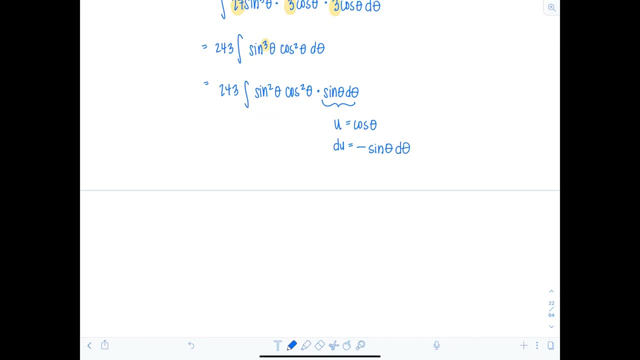 d theta. Okay, no problem. So we've got an extra negative in there. Also, if u is cosine theta, then I want to replace this sine squared theta with one minus cosine squared theta. Okay, so before we make this substitution, let's get everything set up. So we have 243 integral. 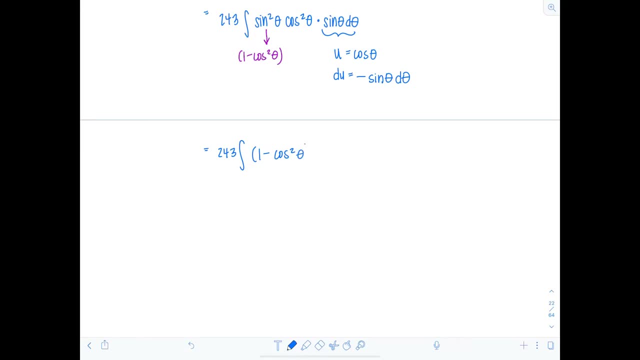 Sine squared theta is getting replaced with one minus cosine squared theta, Then I still have that cosine squared theta. So I'm going to plug off one of the factors of sine squared theta. sitting there and sine theta d theta, Beautiful, All right. so here we go Now. 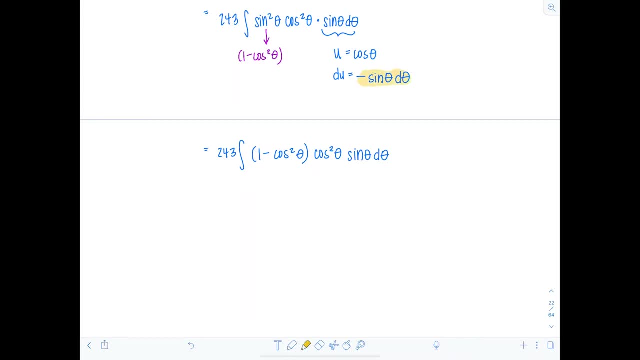 du is negative sine theta d theta. So I'm going to replace this. but I'm going to add a negative in my integral, So I'm going to have negative 243 du, All right, and then one minus cosine squared theta. This is going to get replaced with one minus u squared. 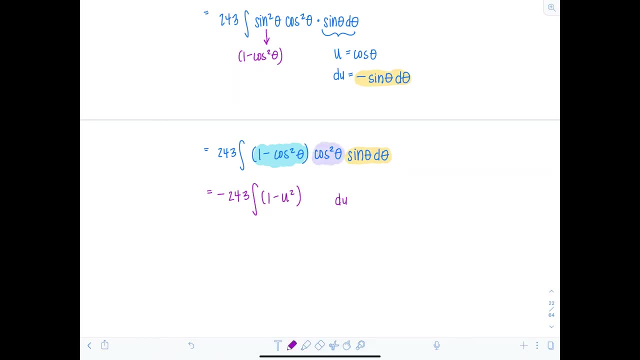 And then cosine squared, theta is just going to get replaced with u squared. Okay, there's that. There's that Color coding it all, so you can see where everybody went. Okay, good, Now let's see How would we deal with this integral. 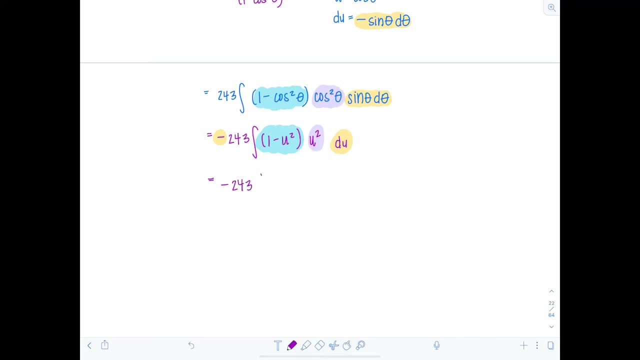 So I have negative 243 times distribute that u squared, So this is going to be u squared minus u to the fourth du. If you want to get rid of that negative, you can reverse the order of subtraction. so this is positive 243, integral u to the fourth minus u squared du. Oh, that looks so much better. 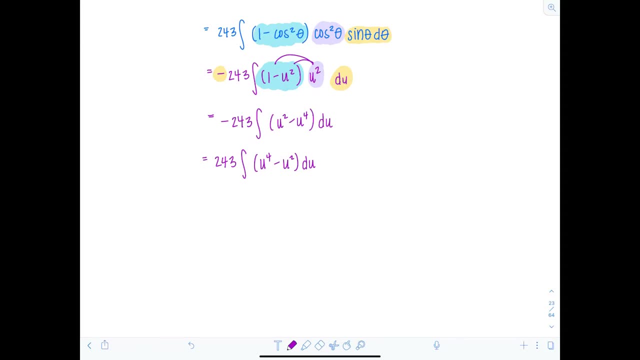 Plus it's in descending order. now, right, Great. And then this is going to be 243 times u to the fifth over five minus u. cubed over three plus c. All right, very good. Now we're going to go back and replace u with cosine theta. 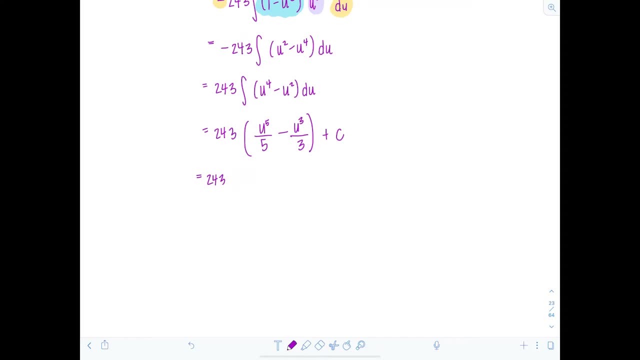 So now I have 243.. This is going to be cosine to the fifth of theta over five minus cosine cube theta over three plus c. Are we done? Should we box it up and call it a day? Uh uh, Remember the original integral was in terms of x. so how do we get back to x-land? 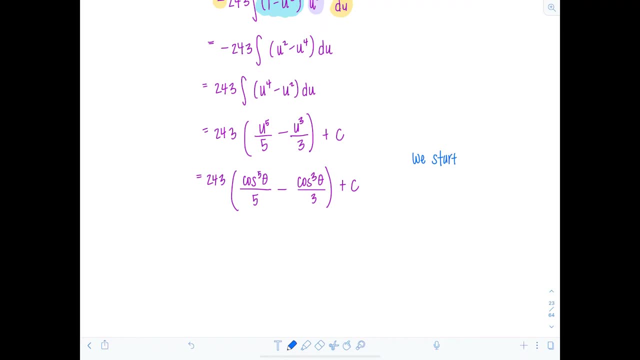 We'll go back to where you started with. We started with letting x equal three sine theta, so I want to replace all of the thetas now, so that everything gets squared. Nice. So we want to replace u with cosine. Come on. 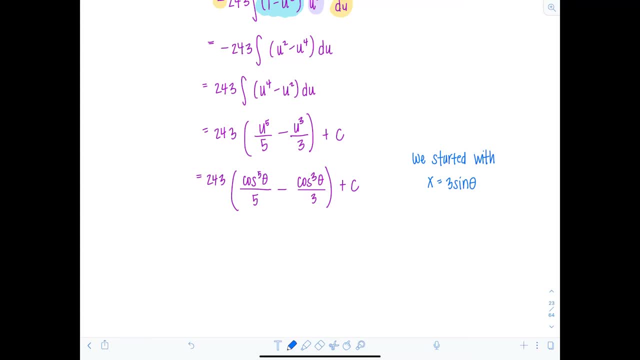 Come on, in terms of x, You have to draw a triangle. Pretend you're in a trigonometry class. So that means x over 3 is equal to sine theta. Let's draw a triangle. Here we go Much better. Here's our right triangle, Here's theta. So sine is the ratio of the opposite. 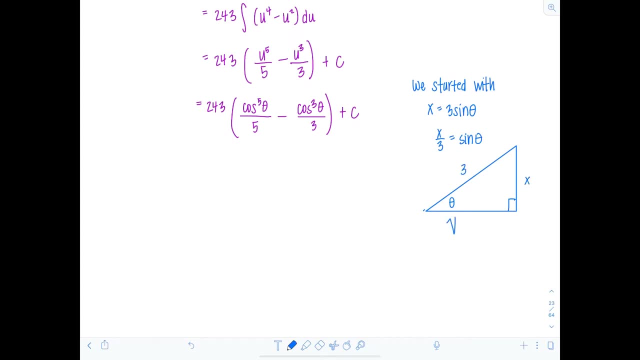 over hypotenuse, and that means the remaining leg is going to be rad 9 minus x squared. Here's a cool tip: The side that you solve for should be the expression that was in your original integral. If not, go back and check something. Okay. well, how am I going to use? 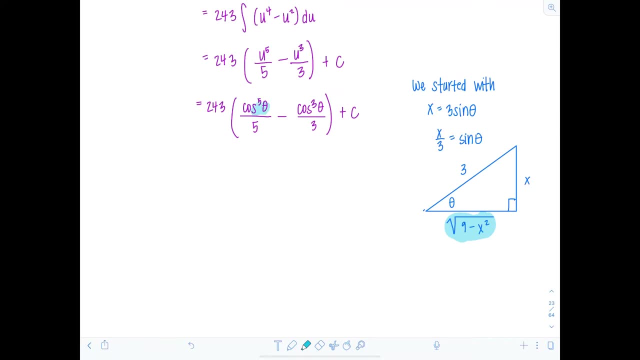 this triangle. Well, can I figure out what cosine of theta is now using this triangle here? I sure can. So cosine of theta is adjacent over hypotenuse. So cosine of theta is going to be rad 9 minus x squared, 9 minus x squared over 3.. Okay, so here we go. Let's sub it all in. So we've got 243.. 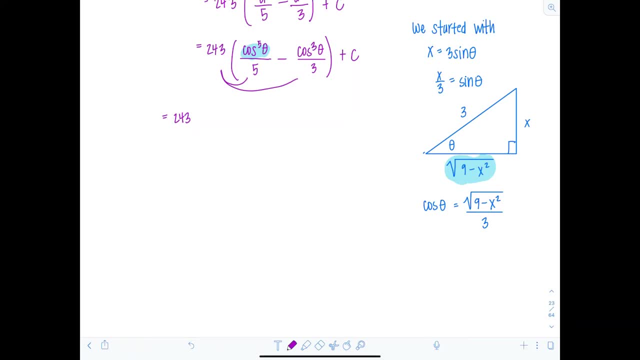 Let's distribute it like this so we don't have to deal. So: 243 over 5, and then cosine of theta, which is rad 9 minus x squared over 3.. This is all raised to the fifth. Okay, So we've got the cosine of theta as rad minus 243 over 3, and then here I have cosine. 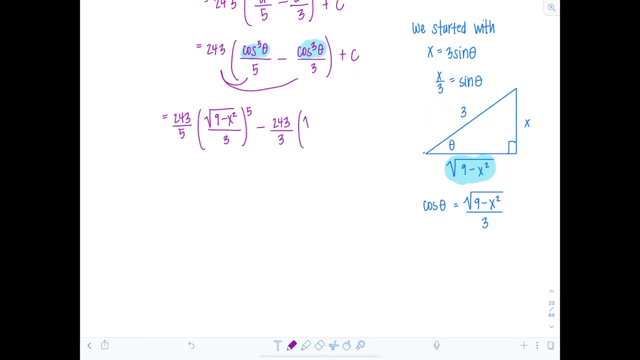 of theta cubed. Okay, so cosine of theta was rad 9 minus x, squared over 3, and now we're cubing this guy plus C. Alright, can we clean it up a wee bit? I certainly hope so. Three to the fifth is 243.. Did you? 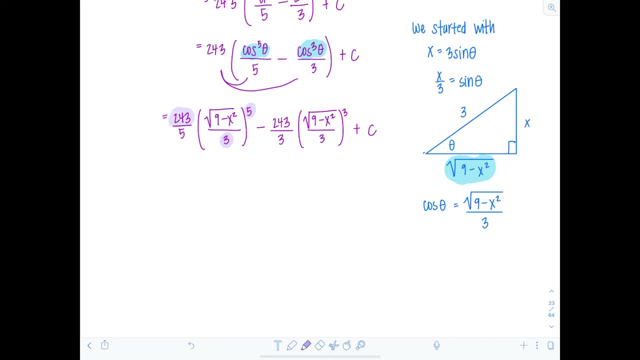 know that. I hope so. If not, you can write that down. you've got a calculator, so you're okay. So 3 to the 5th and 243 are going to cancel out. That's gone. And then you have 9 minus x squared square root of that raised to the 5th. 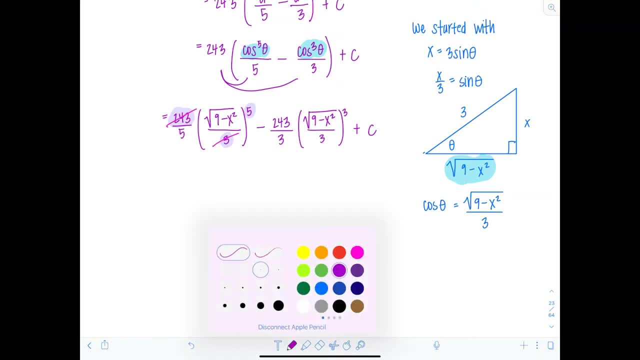 So if you raised it to the 4th power, that would just be 9 minus x squared squared, and you've got one more radical left over. So this is going to be 1: 5th: 9 minus x squared squared times: rad: 9 minus x squared. All right, And then let's see what cancels out over here. 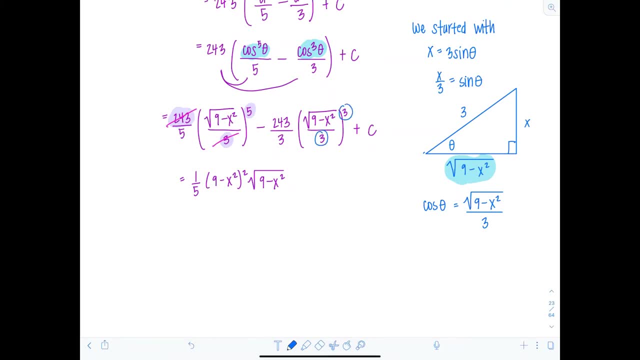 So 3 cubed, that's 27.. And then I've got another 3, that's 81. So 243 divided by 3, divided by 81,- excuse me- is 3.. So I have minus 3.. And then let's think here: If I have rad 9 minus, 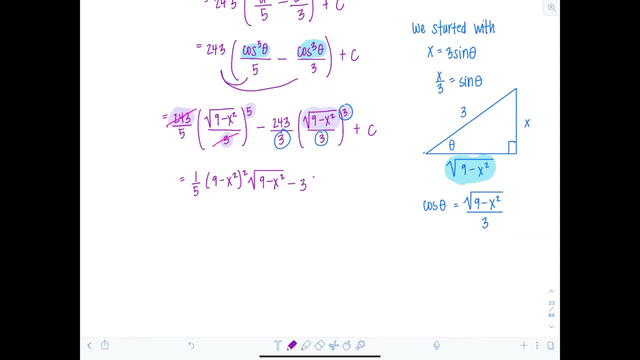 x squared cubed, then I'm going to get 9 minus x squared to the 1st power, and then another rad, 9 minus x squared plus z, And that's your final answer. Okay, let's box it with pride. I mean, that was a labor of love, right there. 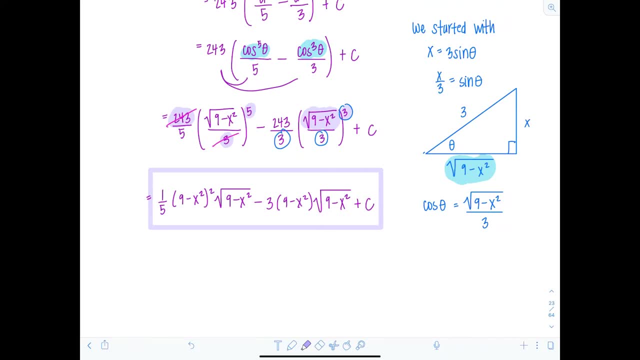 Good. So just be super careful after you use a trig sub. If it's an indefinite integral, you have to go back, Draw that triangle and rewrite everything in terms of the original variable. All right, Good, So that's the first case. Do you remember what it was? a squared minus x, squared. 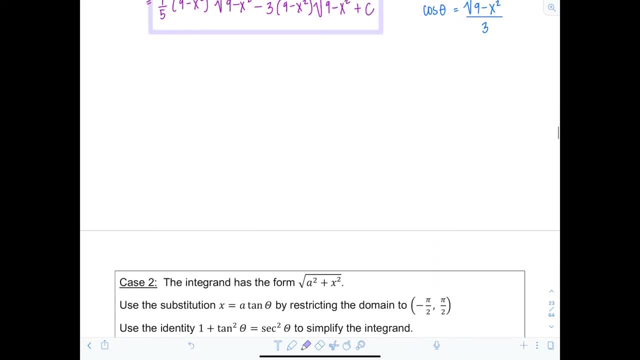 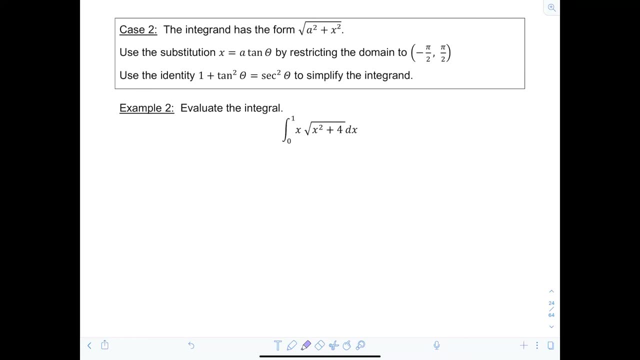 underneath the radical. Okay, case 2.. The integrand has the form radical: a squared plus x squared. Instead of subtraction, it's addition. So you're going to use the substitution x equals a tangent theta- and then restrict the domain and then you're going to have a. 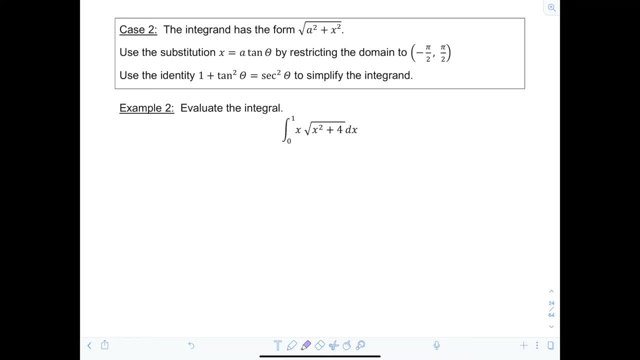 distribution, and then you're going to have a subtraction, and then you're going to have a main on theta to negative pi halves and pi halves not including pi halves or negative pi halves because tangent's undefined there, And then you're going to use the identity 1 plus tangent squared. 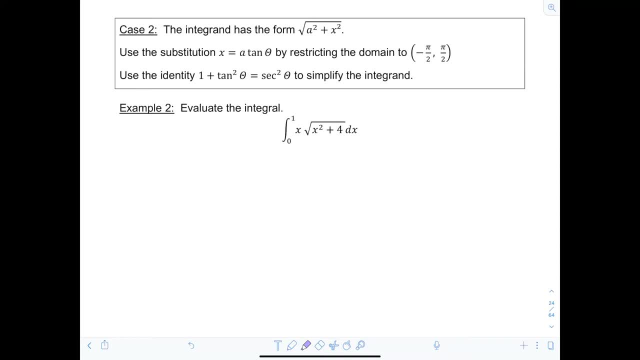 theta equals secant squared theta, to simplify the integrand. Okay, so here we go. We have integral from 0 to 1 of x times radical x squared plus 4 dx. Okay, now I'm going to demonstrate the method of trig sub here. but think about there might be another way to do this integral. 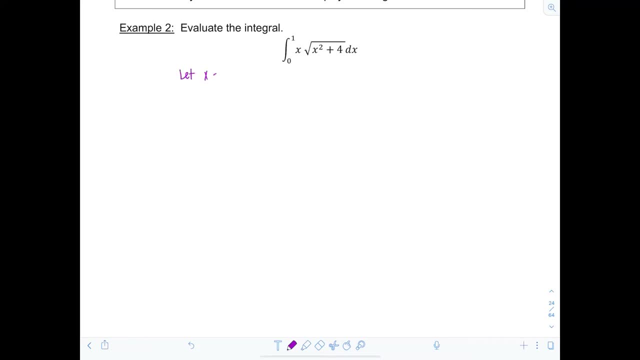 So, starting off, I'm going to let x equal 2 tangent theta right. That's a squared Right here. this 4 is a squared All right. so find dx first. So dx is going to be 2 secant. 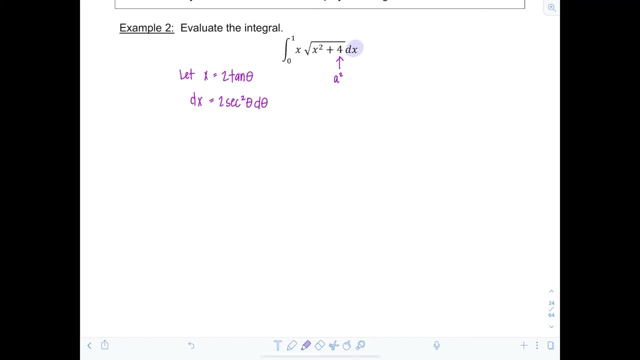 squared theta d theta. So this is taken care of. I'm going to replace it with 2 secant squared theta d theta. Now let's see what's underneath the radical. So we have radical x squared. So that's going to be 4 tangent squared theta plus 4.. And then I can factor out the 4.. 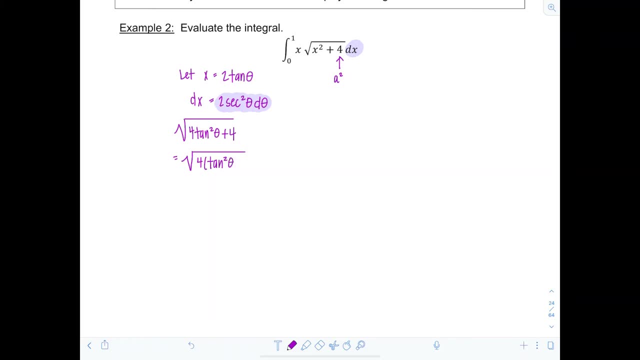 So I have radical x squared, So that's going to be 4 tangent squared theta plus 4.. Radical, 4 times tangent squared theta plus 1, which is going to be radical, for secant squared theta, which is, be careful, do you remember? 2, absolute value of secant theta. 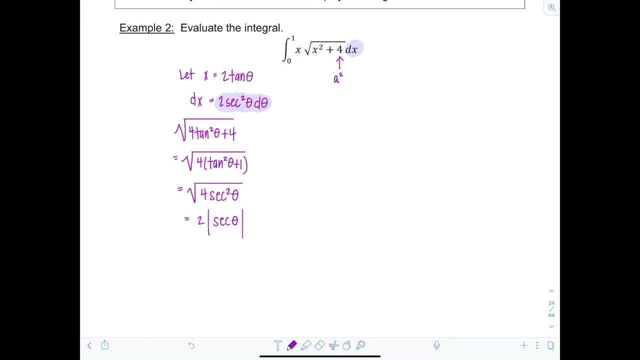 And then, remember, we restricted our angle between negative pi halves and pi halves. So again we're in quadrants 1 and 4. Cosine's positive there, so secant's going to be positive there as well. So we have 2 secant squared theta plus 1. And then we're going to put in the 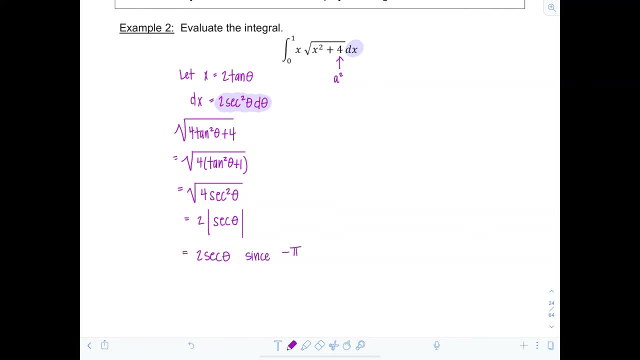 value of secant squared theta d theta, which is 2 secant squared theta d theta. So that's going to be 2 secant squared theta d theta. So that's going to be 2 secant squared theta d theta. So this is going to be 2 secant squared theta d theta. So we know theta is between: 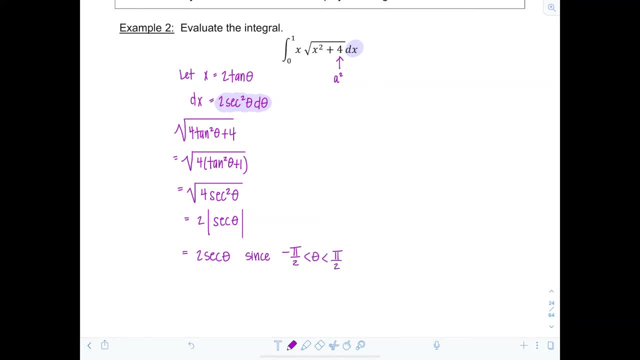 negative: pi halves and pi halves. So now I know I'm going to replace this entire expression here with 2 secant squared theta. In this case I have limits of integration, So I need to figure out what those new limits are going to be in terms of theta. So let's go ahead and be careful you're not plugging. 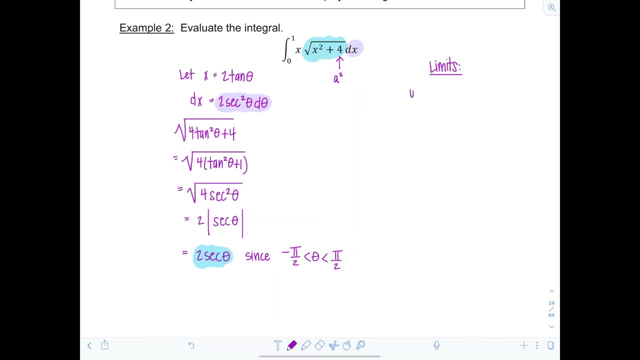 in, you're setting it equal to the value. What do i mean by that? Well, these limits are in terms of x, right? So when x equals 0, remember, x is 2 tangent theta, So that means tangent theta is 0. So what would theta have to be? You're not plugging in 0 for theta. No, no, no. 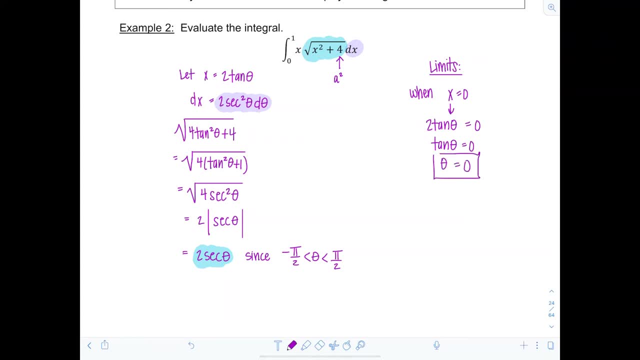 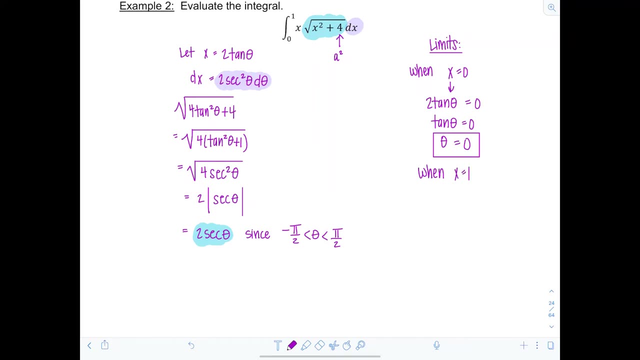 You just think of your unit circle. Theta would be 0. Okay, that one wasn't bad. Now the other limit of 1, when x is 1, that means 2, tangent theta is equal to 1, which means tangent theta is 1⁄2. That's not any nice angle on the unit circle. 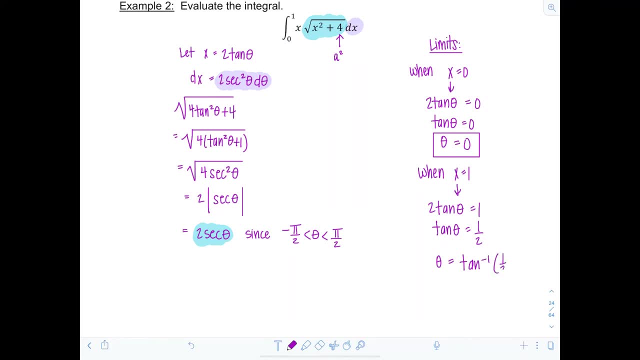 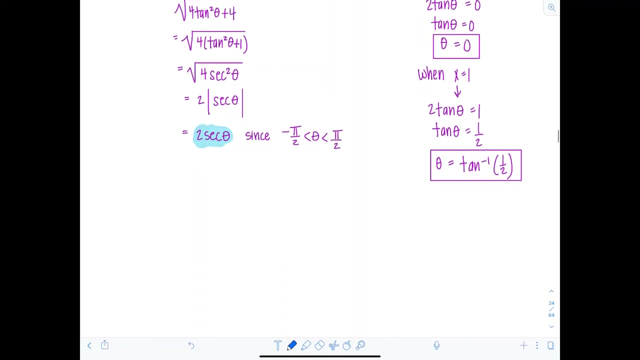 So you're just going to say: all right, theta is tan inverse of 1⁄2. That's our new upper limit. So here we go, Let's switch everything so that it's in terms of theta. So we've got integral. 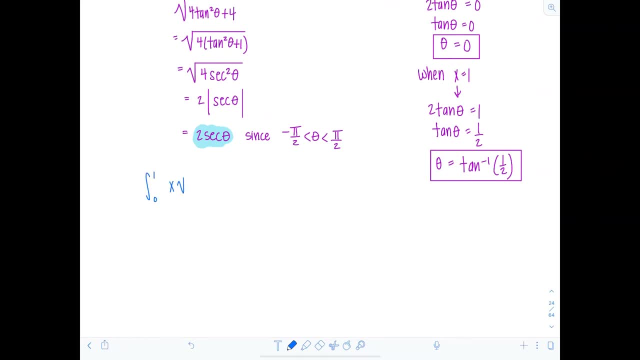 I'll rewrite the original 0 to 1, it was 1.. x times radical, x squared plus 4, dx. Okay so new limits. New lower limit: 0.. New upper limit is tan inverse of 1⁄2.. x gets replaced with 2 tangent theta. 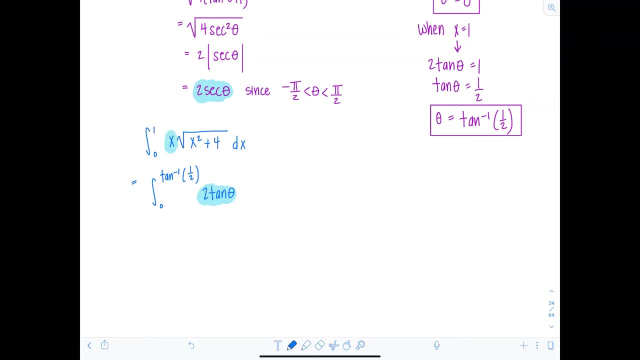 Rad x squared plus 4 gets replaced with 2 secant theta. And then do you remember what dx gets replaced with? We did it first: 2 secant squared theta, d theta. Okay, here we go. Let's see. Take those constants outside, right. 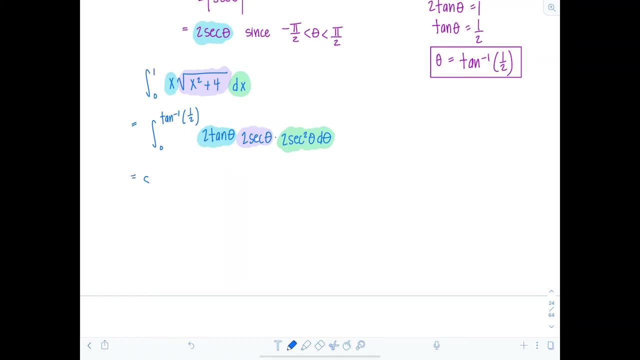 We don't want them bothering us. So I'm going to have 8 integral from 0 to tan, inverse of 1⁄2. And then this is going to be tangent theta times, secant, cubed, theta d theta. Do you remember this case? what you're supposed to do? 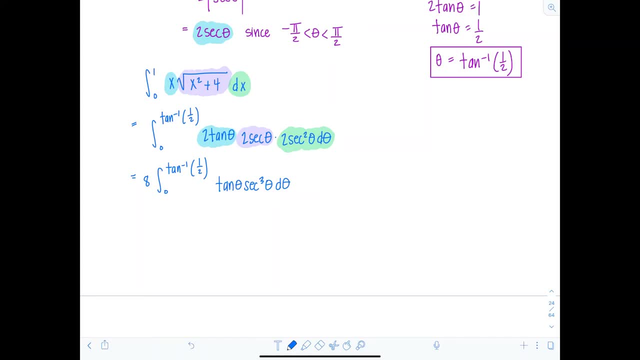 You're going to pluck off one factor of tangent, one factor of secant, so you can make a? u substitution. So this is going to be 8 times the integral 0 to tan inverse of 1⁄2.. And then I'm going to take off one factor of tangent, one factor of secant and one factor of secant. 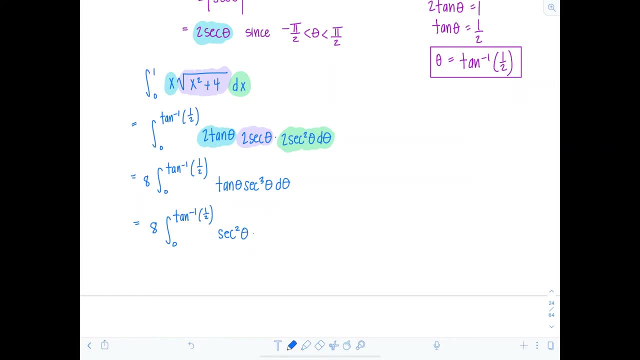 So I'm going to be left with secant squared theta times tangent theta, secant theta d theta. Why do I do that? Because I want this to be absorbed in my du, which means I would need to let u equal secant theta. 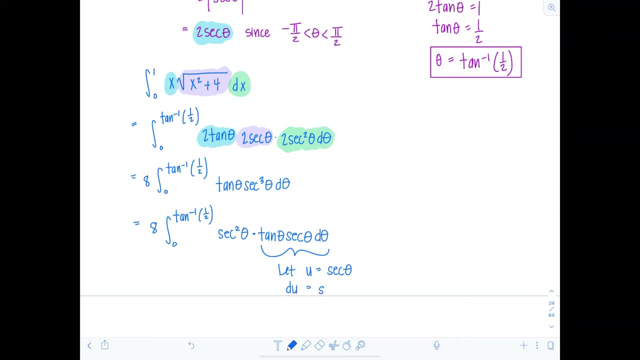 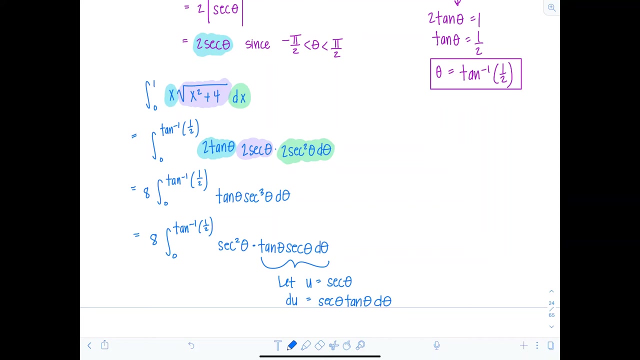 And then du would be secant, theta, tangent, theta d theta. All right, Very good. Okay, from here let's figure out what our new limits of integration are going to be. if I change this whole integral to be in terms of u. 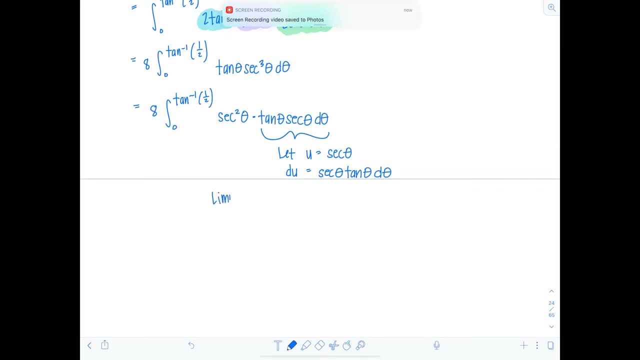 Okay, So the limits u of I'm going to. now I plug it in right. This is a different substitution, So u of 0 is equal to secant of 0, which is which is 1.. And then u of tan inverse of 1⁄2. 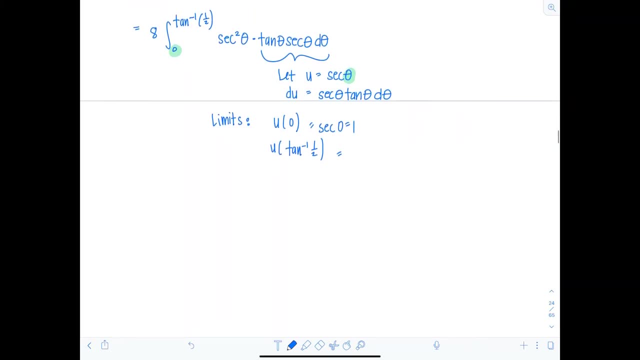 My goodness, how do you do that? So that's going to be secant of tan, inverse of 1⁄2.. And then you think back to trig days, precalc days. Yes, it's triangle time again, Woohoo. 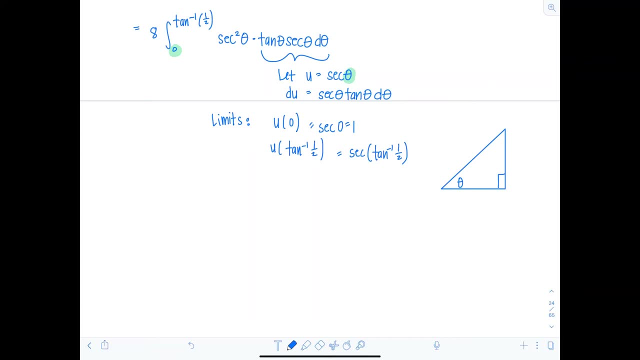 So here we go. This represents some angle, right? This is my theta. So tangent of theta is 1⁄2, which means ratio of opposite over adjacent is 1⁄2.. Hypotenuse is going to be rad 5.. 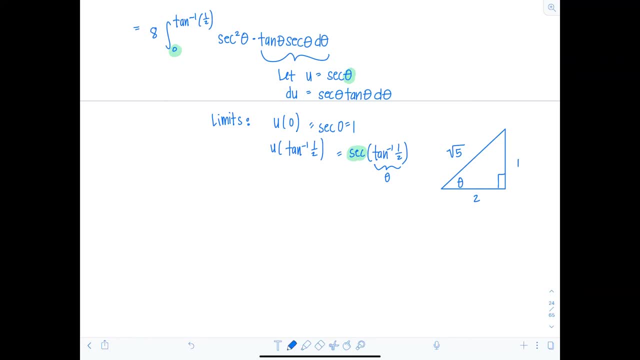 Now can you figure out what secant of that angle is? Secant's going to be hypotenuse over adjacent, So that's going to be rad 5 over 2.. And there you go, There's your new upper limit. 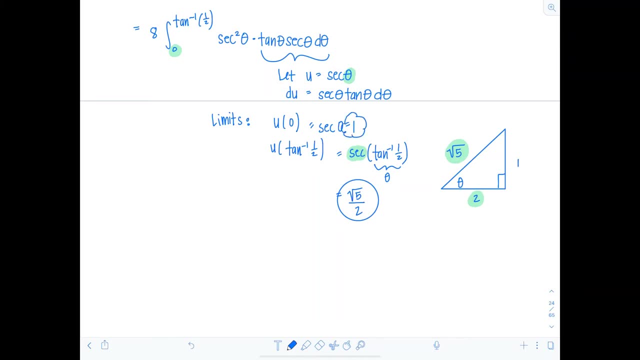 New upper limit, new lower limit. See how important trig is. Okay, So let's rewrite our integral now all in terms of: u, The 8 just comes along for the ride. Sit tight, 8.. Here we go. So we've got 8 integral 1 to rad 5 over 2.. 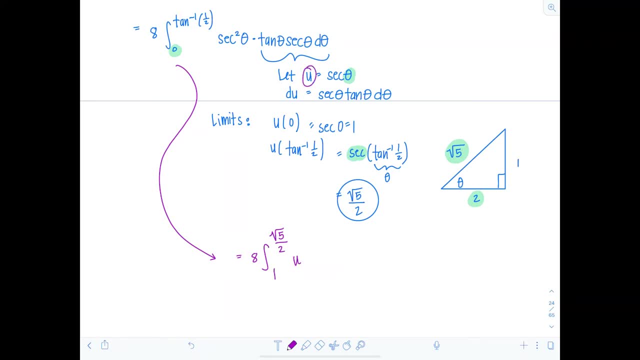 Secant squared theta. That's just going to be u squared, And then tangent theta, secant theta, d theta is du Woo. The worst is over. Look at this cute little integral. We got this, No problem. Add 1 to the exponent. 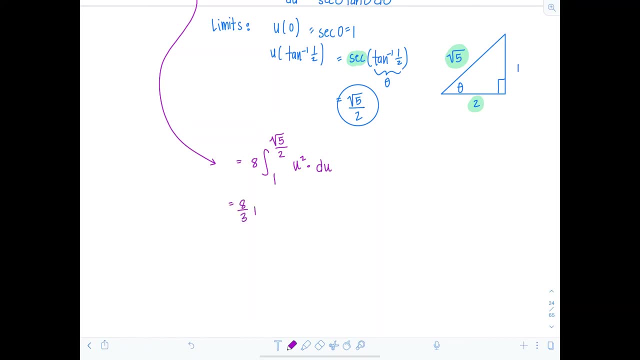 Divide by the new exponent, This is 8 thirds u cubed, evaluated from 1 to rad 5 over 2.. Okay, Okay, So we've got 8 thirds times rad 5 over 2 cubed, minus 1 cubed. 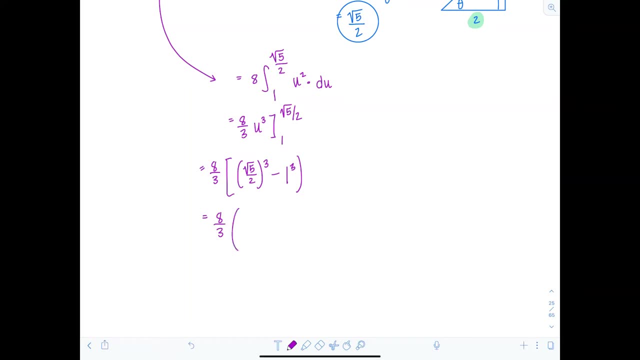 So this is 8 thirds times rad 5 cubed, That's going to be 5 rad 5.. 2 cubed is 8 minus 1.. And then let's distribute the 8 thirds, because it's going to cancel so beautifully, right. 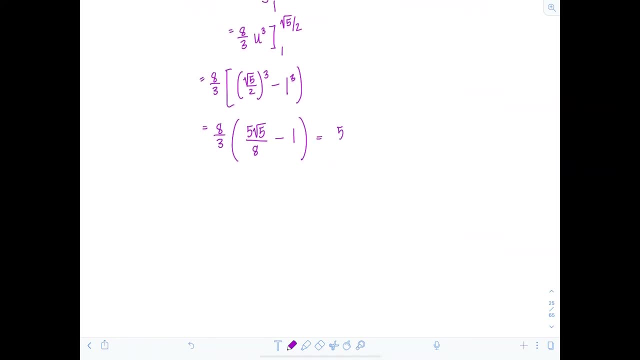 So we'll have for our final answer 5 rad 5 over 3 minus 8 thirds. So 5 rad 5 minus 8 over 3.. And we are done Fabulous. Did you ever anticipate trigonometry to come back with such a vengeance in calculus? 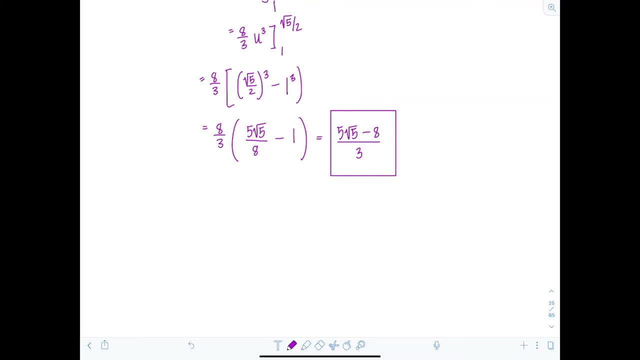 All right, Let's look at another example with this same case. that's a little more fancy. Okay, It's time to kick it up a notch. So we're going to evaluate the integral And I've put in a nice little hint for you. 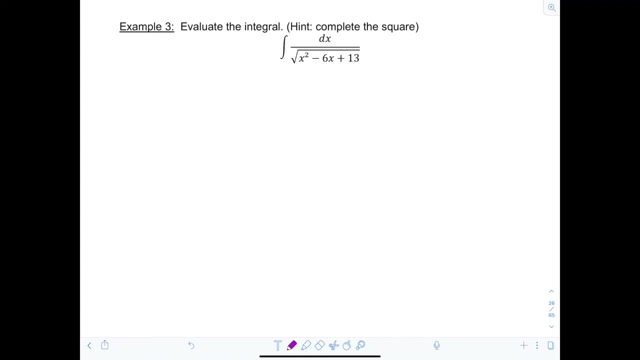 You need to complete the square, The square underneath the radical. that way you could have the form x squared plus a squared right. So do you remember how to complete the square? If you have x squared minus 6x, what constant would I need to have a perfect square trinomial? 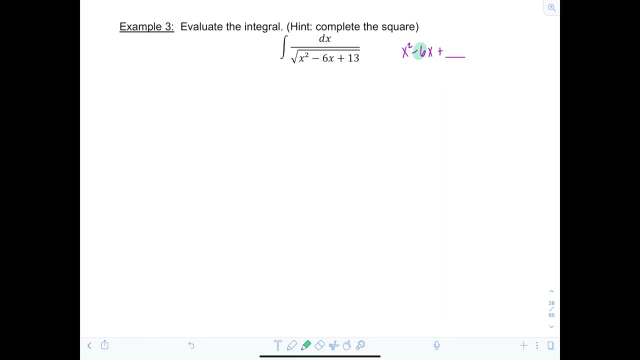 You take the coefficient of the linear term, divide it by 2, and then square it. So I would need to have a 9 in order to be able to factor this into x minus 3 squared. Okay, Well, notice here, this is 13.. 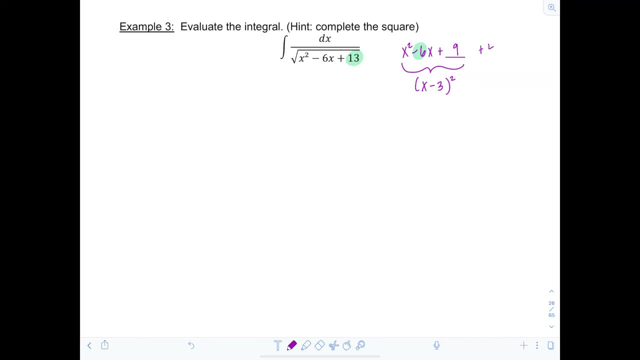 So I'm just going to steal 9 away And then I have plus 4 left over. Oh my, that's convenient, right? So I can let x minus 3, just treat that as one whole quantity, right? Instead of x, now we have x minus 3 equal 2 tangent theta. 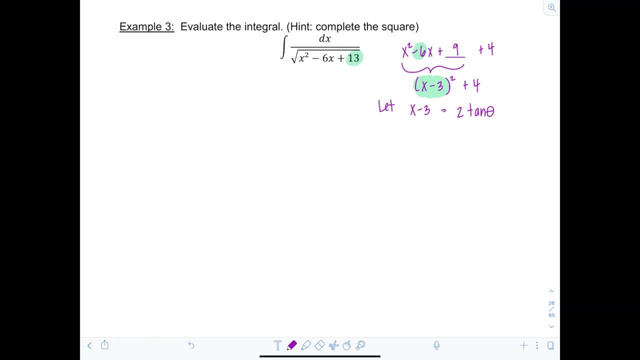 So a is going to be 2.. You see that It's a little different than before, But the rest of it just falls into place the same way. So you're going to find dx. Derivative of that negative 3 is 0.. 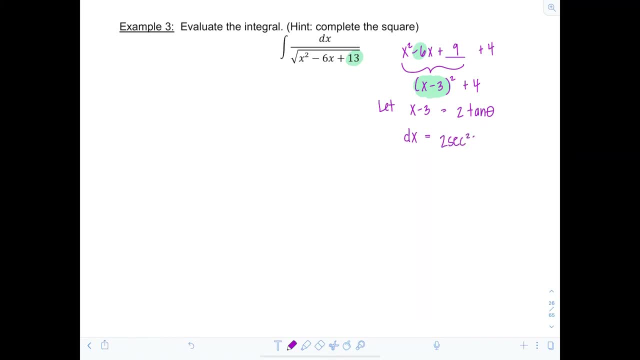 So you're just going to get dx equals 2. Secant squared: theta d theta. See, No big deal, Okay. So now let's go ahead. see what's going to happen in our integral. So we have integral of dx. 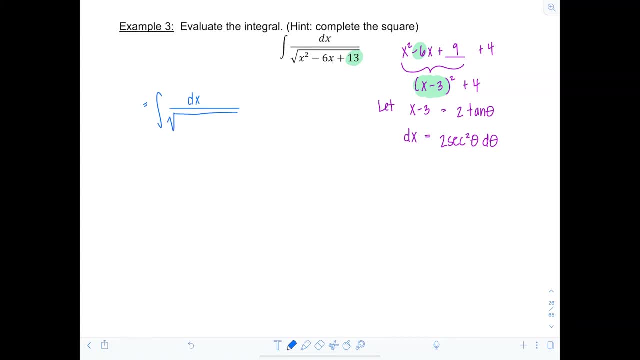 I'm first going to rewrite the denominator as radical x minus 3 squared plus 4.. Okay, So dx, in the numerator It's going to get replaced with 2 secant squared theta d theta, And then in the denominator we have that rad x minus 3 squared. 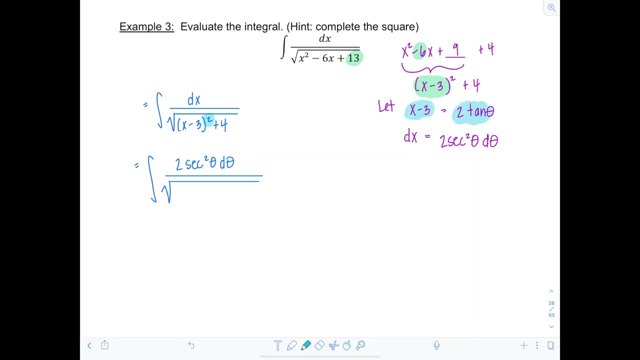 So if I square x minus 3, I'm going to square 2 tan theta, So that's going to be 4 tan squared theta plus 4.. All right, And then, remember, I can factor that 4 out And then I have tangent squared theta plus 1.. 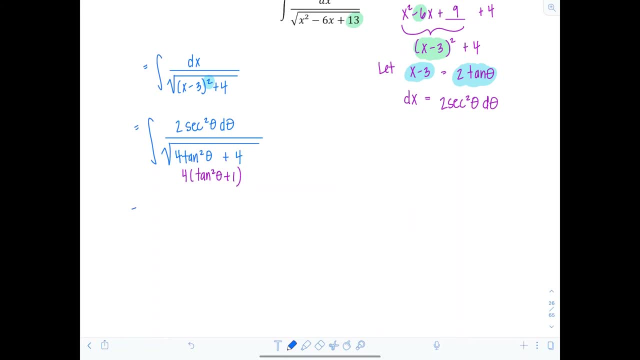 Good, good, good. So next step, let's clean up a little more. We've got integral 2, secant squared theta, d theta over radical 4.. And then now I can replace tan squared theta plus 1 with secant squared theta. 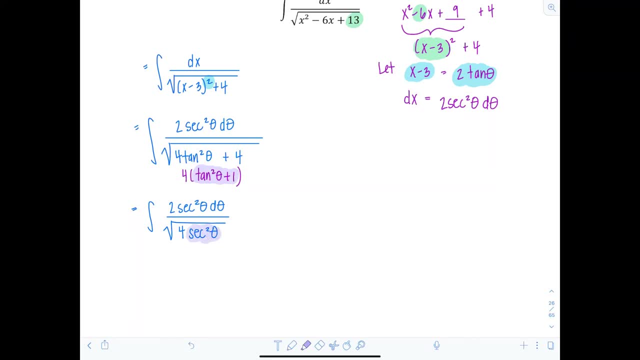 Okay, And then remember- this is going to simplify for us- I've got 2 secant squared theta d theta over it's 2 absolute value secant theta. But we know we're going to choose the positive because we restricted theta. 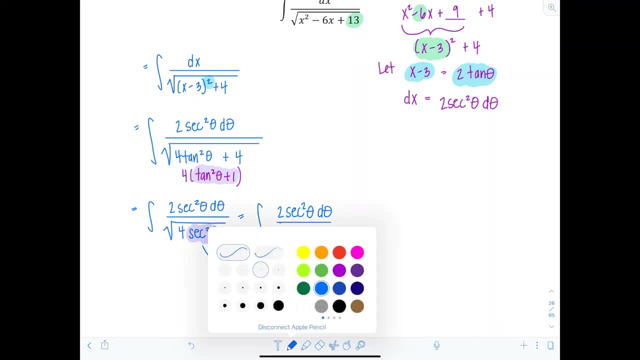 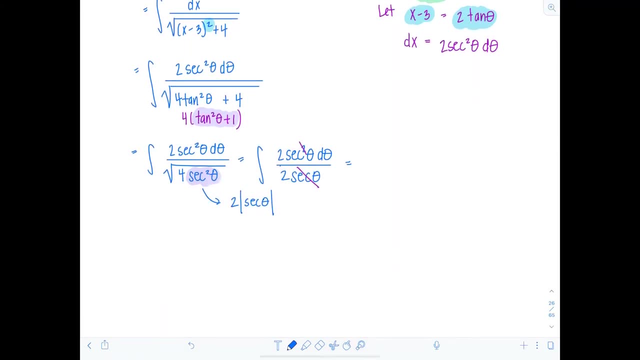 So I just have secant theta and a 2 in the denominator. One of them is going to cancel, Cancel out, And then you just have the integral of secant theta, d theta Right, And the 2 cancels as well. 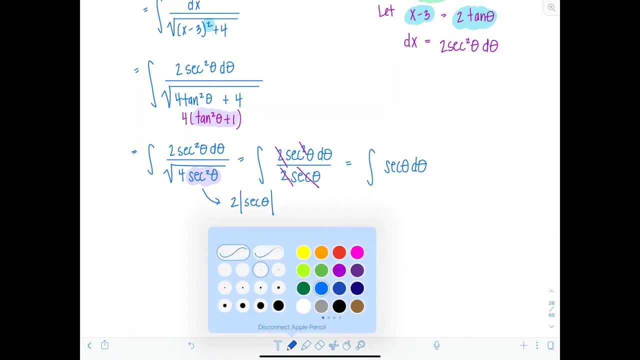 Do you remember what this is? I told you to memorize it just because it's going to come up so often and you don't want to have to do that funky little u substitution every time to remind yourself. You probably won't remember how to do it if you don't even remember what the integral is. 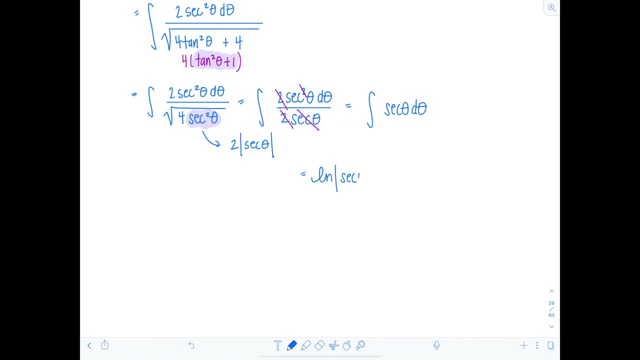 So it's natural log Absolute value: secant theta plus tan theta plus c. Are we done, Surely? I feel like this problem has gone on long enough. No, no, no, The original integral was in terms of x, So I have to rewrite everything with respect to x, in terms of x. 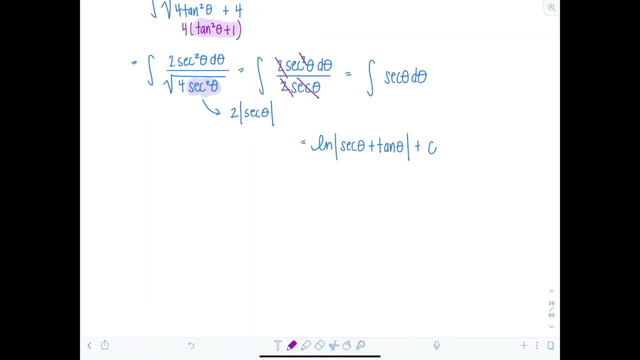 So here we go, Go back to the original substitution. Remember we let x minus 3 equal 2 tan theta, Which means that tangent of theta equals x minus 3 over 2.. So it's triangle time. Here's theta. 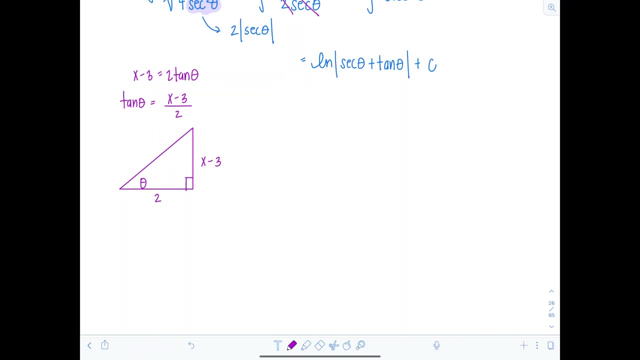 Tangent is going to be ratio of opposite over adjacent, And that means the hypotenuse is going to be rad x minus 3 squared plus 4.. Which we know. before we completed the square, It was x squared minus 6x plus 13.. 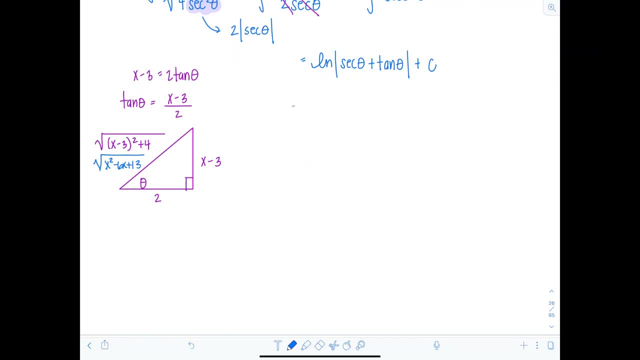 Okay, So now I'm going to come back to the integral. Replace everything. So it's in terms of x, So secant of theta. That's going to be the ratio of the hypotenuse over the adjacent side. So that's going to be radical x squared minus 6x plus 13 over 2.. 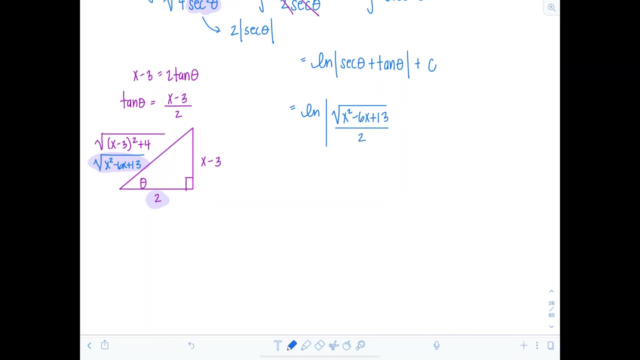 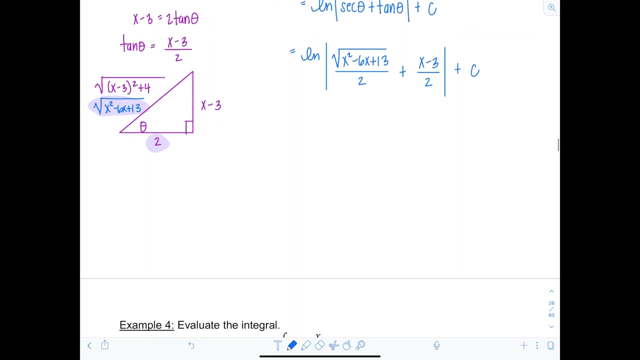 plus and then tangent theta. I already have that. That's x minus 3 over 2 plus c. Okay, you're not done. You can clean this thing up, and it's important that you do so. So notice, I can write these with a common denominator. So I have ln absolute value, radical x squared minus 6x. 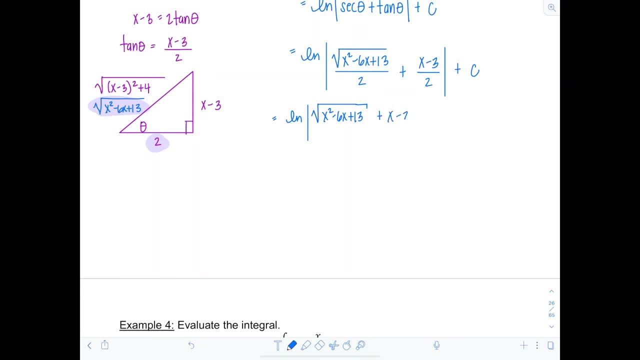 plus 13 plus x minus 3, all over 2 plus c. and then you can use your properties of logarithms and rewrite this as natural log: absolute value: radical x squared minus 6x plus 13 plus x minus 3, and then I'm going to subtract the natural log of 2. 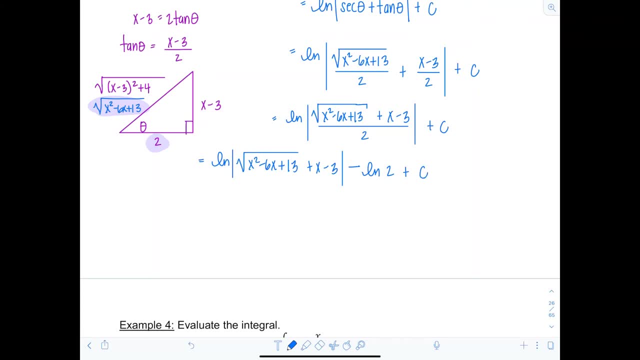 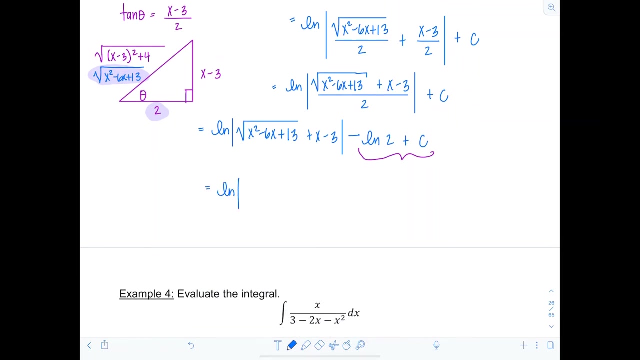 plus c And really natural log of 2 is just a constant, so I can absorb it with the plus c and have a much cleaner expression. So make sure you do this and this is just going to end up being natural log. absolute value radical x squared minus 6x plus 13 plus x minus 3 plus d, where 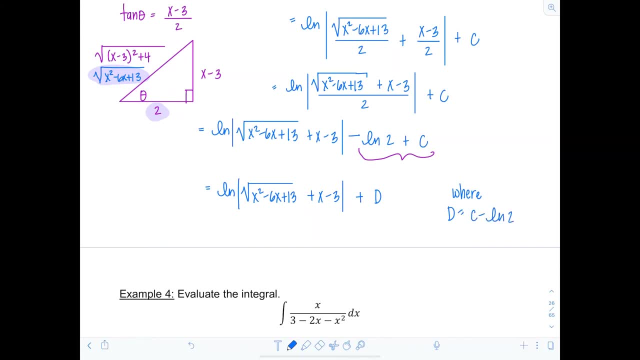 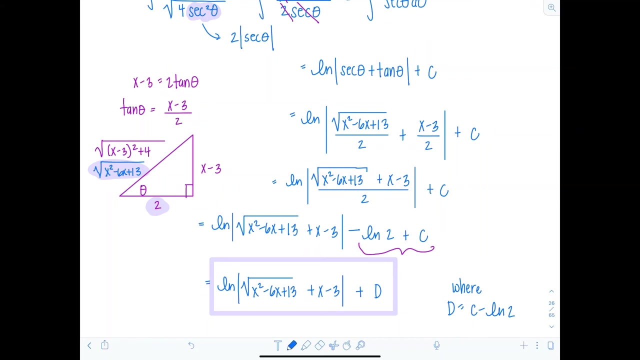 d is equal to c minus natural log of 2.. So when you check your answers, typically it'll just have this cleaned up version, but they'll probably swap out d with c. So if you want to do it so that yours also has a c at the final step, all you would have to do is change it earlier. 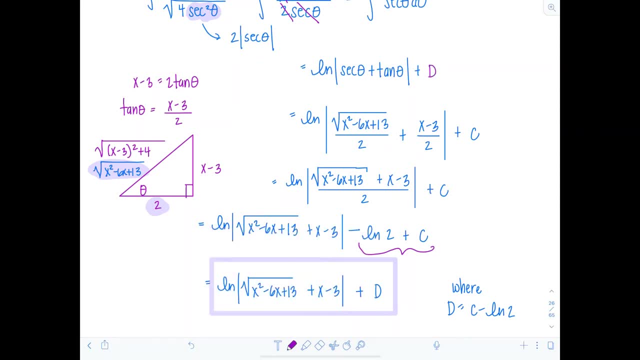 So you could say: call that instead d, d, d or whatever you want, And then this: make a C. if it bothers you that it's not C at the end, It doesn't matter, It's just plus a constant. You just got to remember to do that. Okay, I'm leaving it alone, It's good. 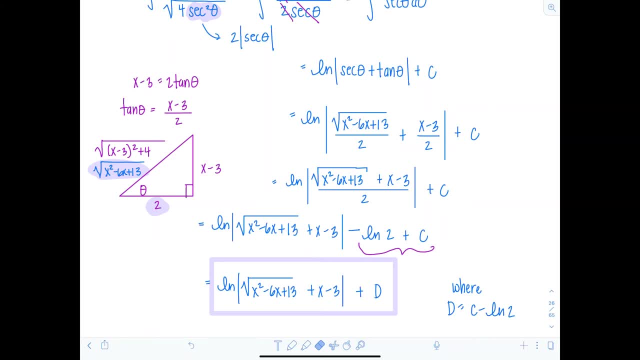 All right, Let's look at another one where we need to complete the square before we move on to the third and final case, And I want to demonstrate this one because I did mention at the very beginning that sometimes you'll use these trig subs even if there isn't a radical. 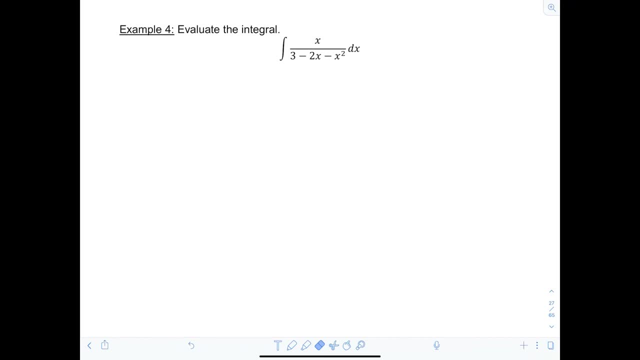 Right. So even if there isn't a radical, I'm looking at this and I've got this quadratic expression in the denominator and it's not looking like a U-sub is going to help. You always want to see if I can do a U-sub first, because that's the easiest, most straightforward. 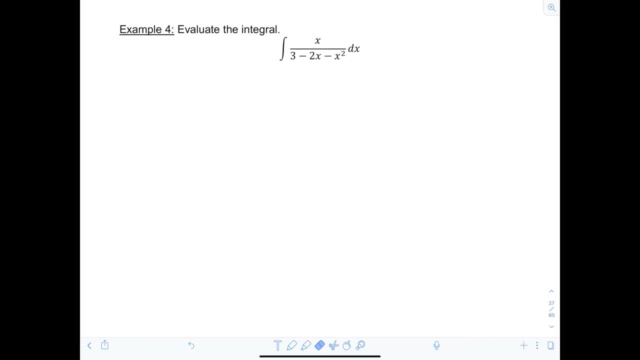 way to anti-differentiate. But if it doesn't, then you have to get out your more fancy tools. Okay, Can we complete the square for 3 minus 2x minus x squared? It's a little tricky. You got to factor that negative out of the x's, So when you have 3 minus, 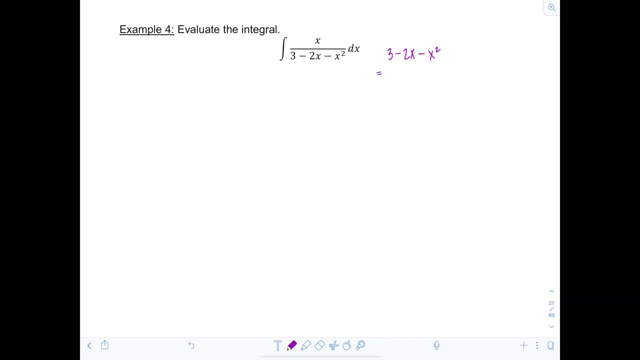 2x minus x squared. you're going to rewrite that as 3 minus. I'm going to have x squared plus 2x And then, remember, divide the linear terms coefficient by 2 and then square it. So I'm going to add 1.. But really that's a negative 1, isn't it? Because of this minus sign sitting. 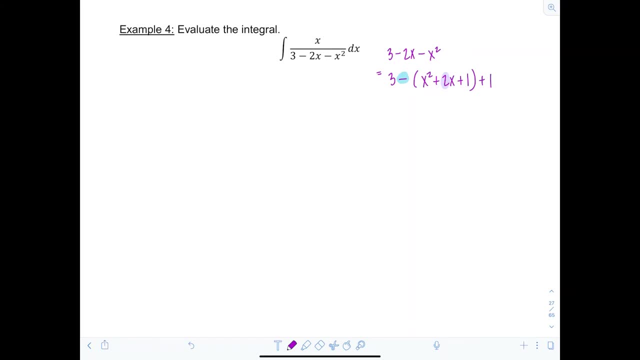 out here. So now I have to add positive 1 to compensate. So combining my constants together, now I have 4 minus X plus 1 squared. Beautiful, Okay. this is the first case that we looked at right Using sine When you have. 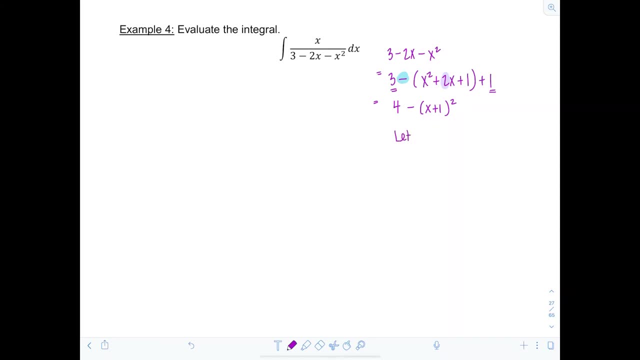 a squared minus a variable squared. So I'm going to let x plus 1 equal to sine theta, And then dx is going to be 2 cosine theta, d theta. Okay, So let's go back to our integral. Now we have 3 minus 2x plus 1 squared, So that's a negative 1,. 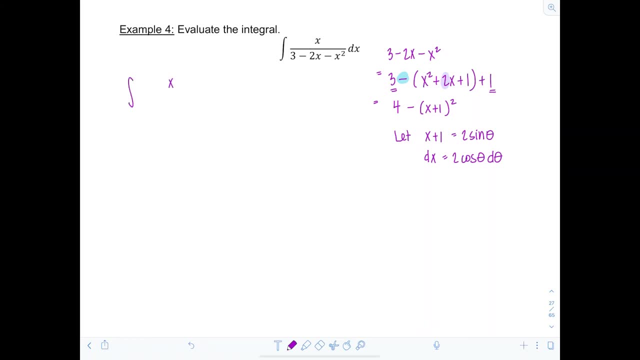 so we're going to add negative 1.. But really that's a negative 1, because we're going to add negative. We have x plus 1 squared, have integral of x over. I'll replace the denominator now with 4 minus x plus 1 squared. 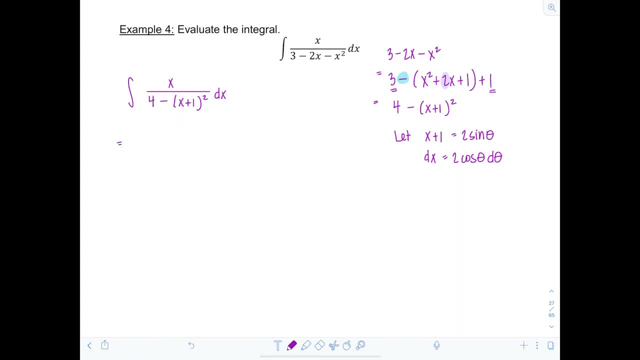 dx. Okay, so in the numerator I have just a plain old x, So that's going to get replaced with 2 sine theta minus 1.. Do you see that? Be careful. And then in the denominator 4 minus x plus 1, squared, that's going to be 4 minus x plus 1 was 2 sine theta. So this: 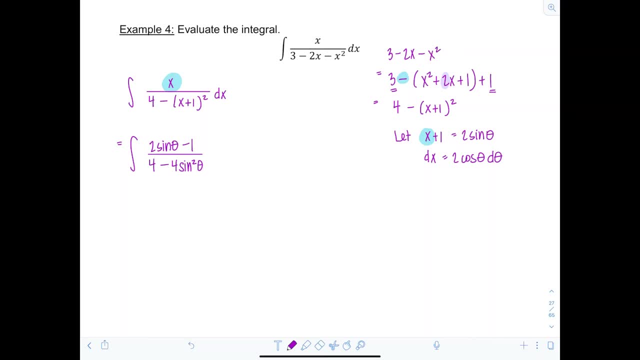 is 4 sine squared theta, And then dx. over here, dx is going to get replaced with 2 cosine theta d theta, 2 cosine theta d theta. Good, All right, let's see What cleaning up can we do. So we have integral 2 sine. 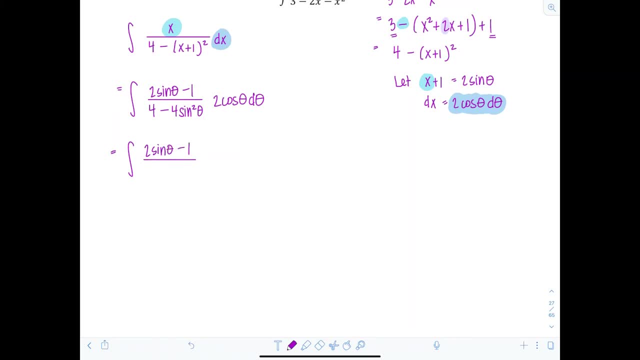 Theta minus 1 over 4 minus 4 sine squared theta, That's 4 cosine squared theta. And then here's 2 cosine theta d theta. So I can cancel out a cosine. That's good. I can also cancel out this 2.. And now the 4 in the denominator becomes a 2.. Okay, so let's split this up. 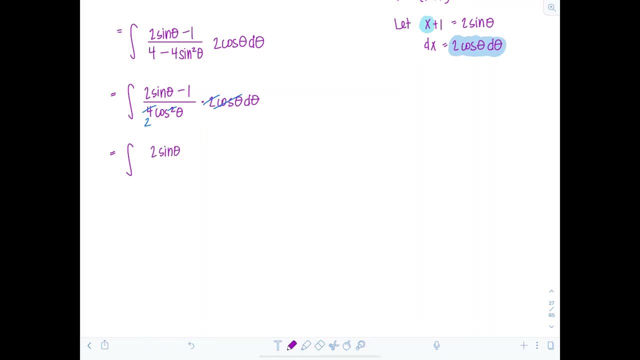 Notice we've got 2 sine theta minus 1 in the numerator. Then I have 2 cosine theta in the denominator d theta And a u sub won't work, Like if I were to let u equal cosine theta. du would be negative sine theta. But what would I do? 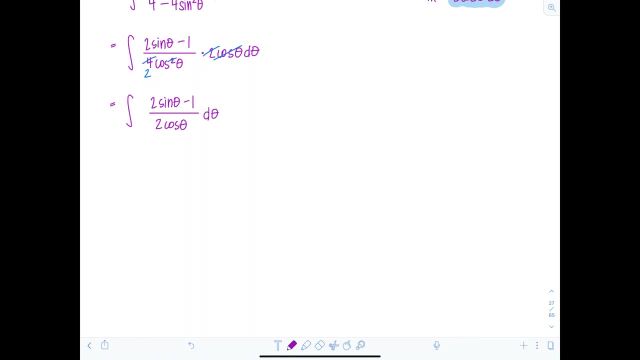 with that minus 1? I'm stuck. So I'm going to split this integral. split the numerator like this: I'll have 2 sine theta over 2 cosine theta minus 1 over 2 cosine theta. So I'm going to do this. 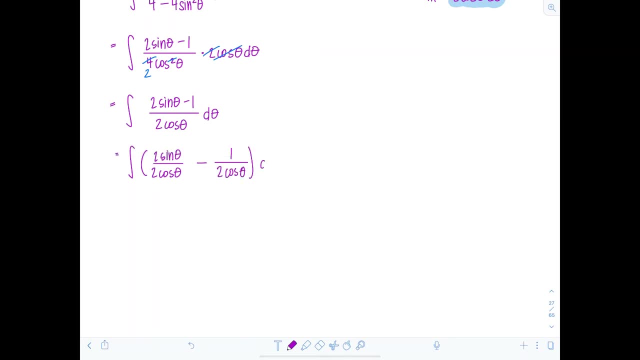 2 cosine theta, And then you have just d theta hanging out there. still, Don't ever forget it, Especially because now we're so fancy, right, We go dx to d theta to du All in one problem sometimes. Okay, this is looking good because now I have integral. These 2s are going to cancel. So 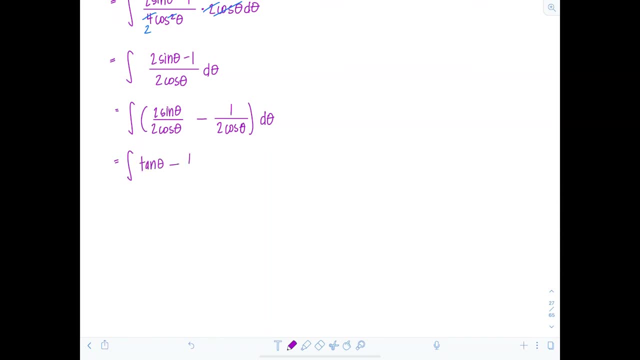 I just have tangent theta minus 1 half secant theta d theta. Do we know these antiderivatives? No, No, No, No, I hope so. So antiderivative of tangent theta natural log absolute value, secant theta. 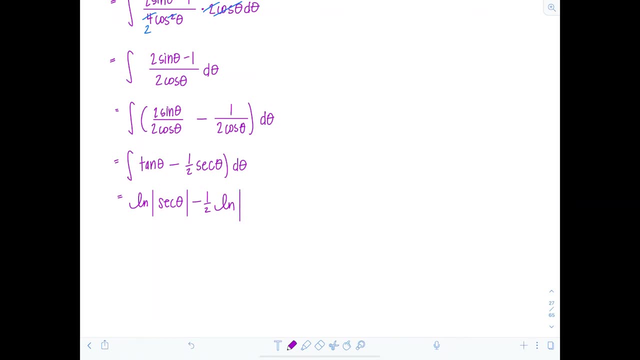